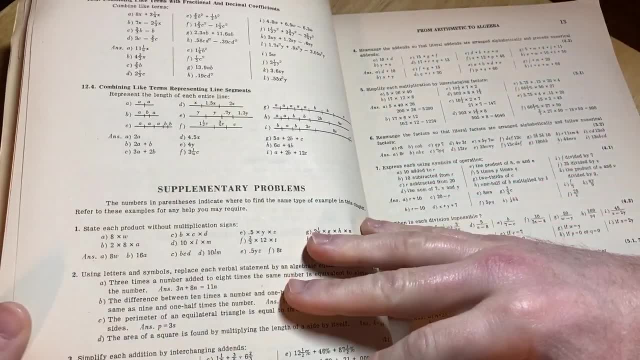 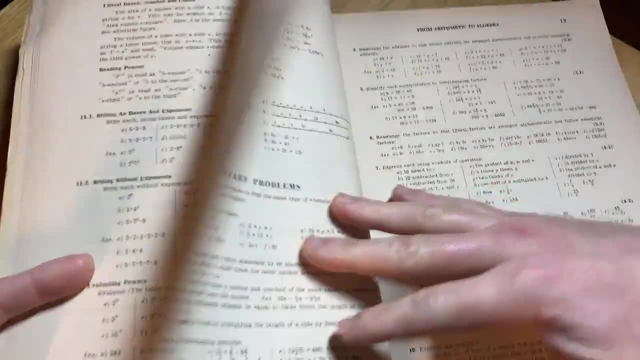 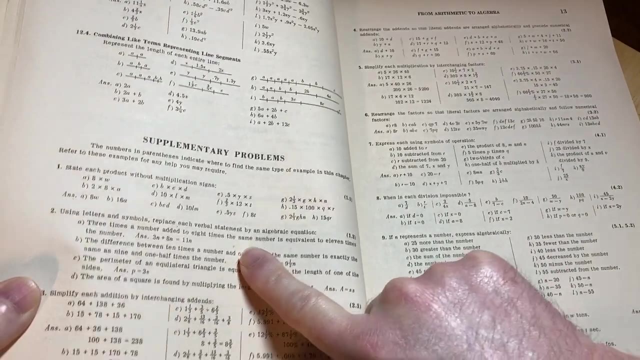 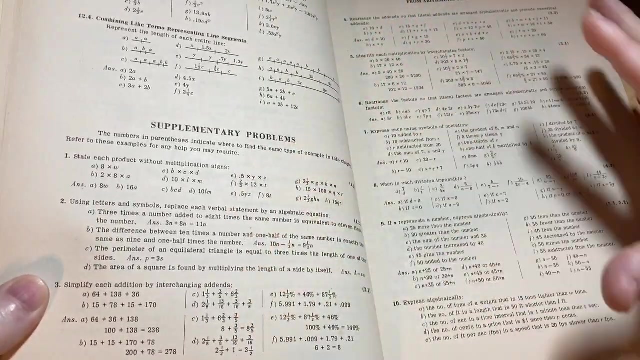 But the idea is the same. You have examples and exercises and just lots of examples. You have some information and lots of examples And then here you have supplementary problems And notice you have answers to them. right, They give you the answers to the problems right next to the supplementary problems. So that's really really good. Depending on the Sham, sometimes the answers will be after You'll have all the questions and then the answers. Sometimes you'll have the answers in the back of the book. 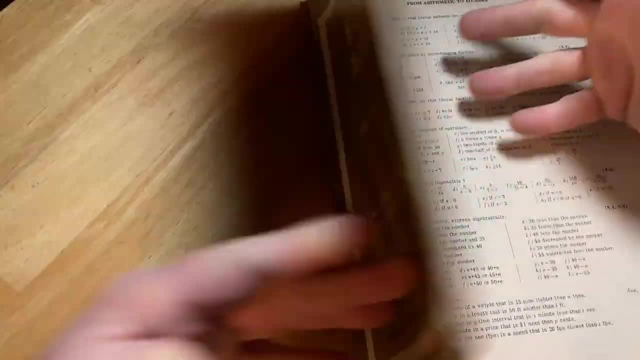 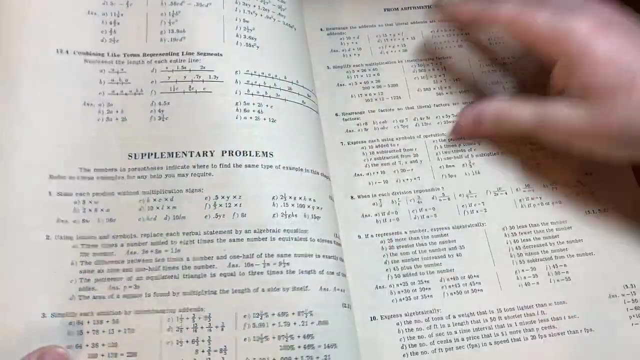 case, you have the answers right here with the exercises. so that will vary from Shams to Shams, right? this is the Shams outline series, and so they have a bunch of algebra books, so this is just one of them. this is the elementary algebra one, which seems to be very, very good. and then here's chapter two, simple. 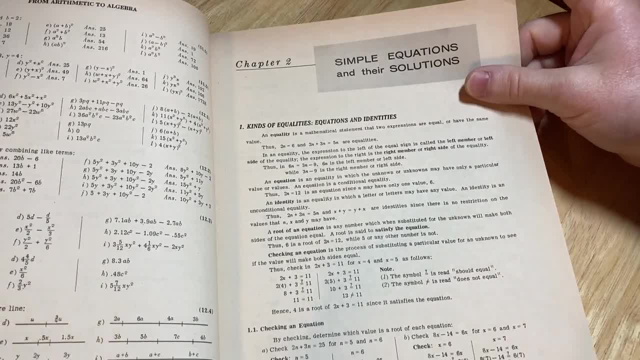 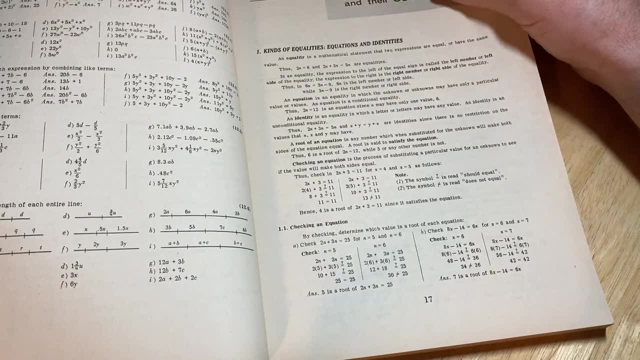 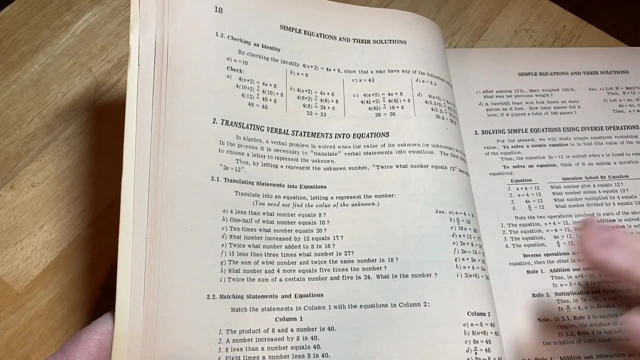 equations and their solutions- kinds of inequalities, equations and identities- cool. so checking equations, that's pretty easy, right, you just take your answer and plug it back into the original and, if it's true, then you verified your solution. translating statements into equations: okay, that's useful. inverse operations: yeah, you can do a lot of word problems with that with the translation. 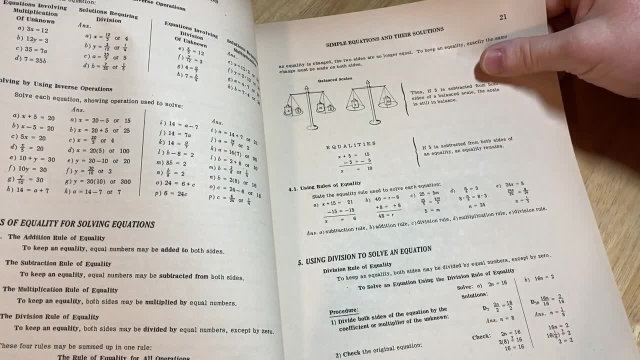 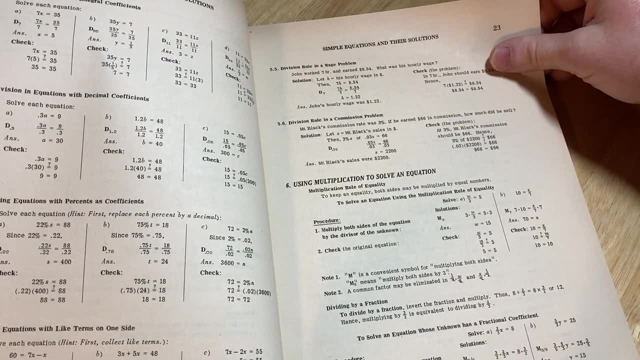 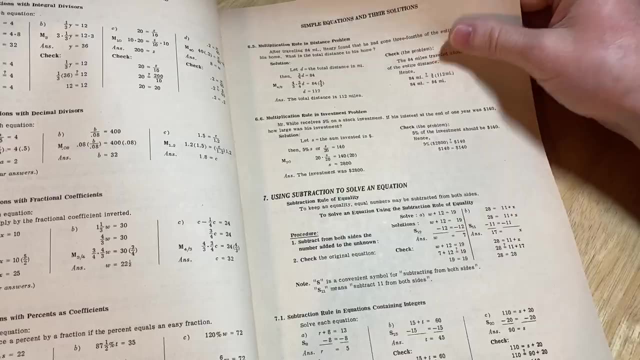 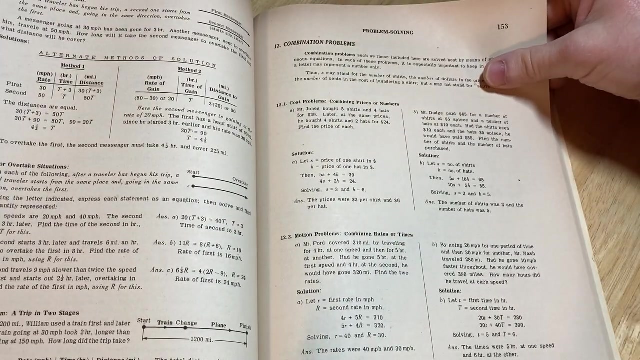 of sentences into equations and stuff. a lot of like basic algebra word problems can be done that way, mm-hmm, pretty cool, simple equations using subtraction to solve an equation. so yeah, tons of mathematics in this little book- a big book actually, I shouldn't say little combination problems, Wow, Wow. oh, this is a little bit different, not what? 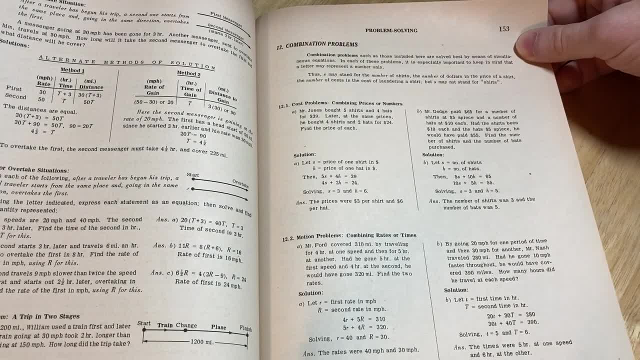 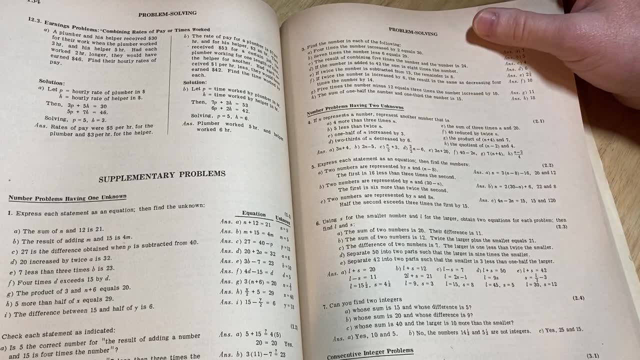 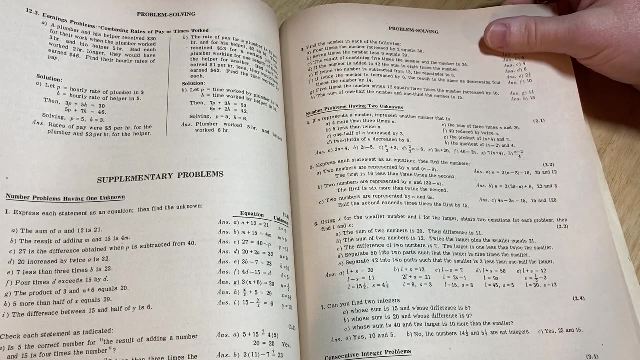 I expected, solve by simultaneous equations. that's what they mean by combination problems. okay, not like problems involving combinations. a combination is a selection that you take from something you know without regard to the order, so like if you have three people and you want to pick two, you know. 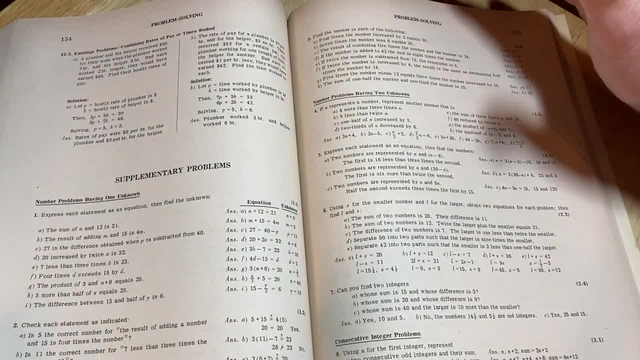 if you have Bill, Joe and Sally and you pick two people and you pick two people, you're gonna be picking Billhole, though we pick your bill. doesn't matter which one you pick first, you're still picking those twos. so it's like you're picking. 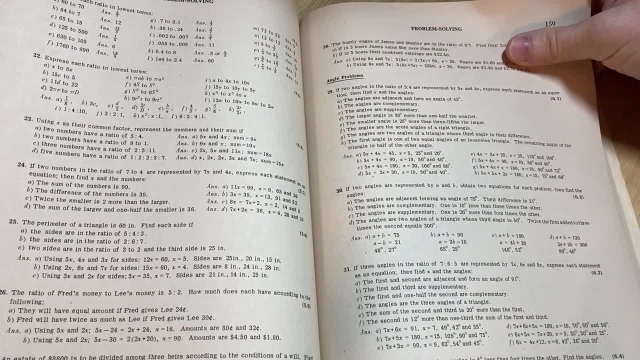 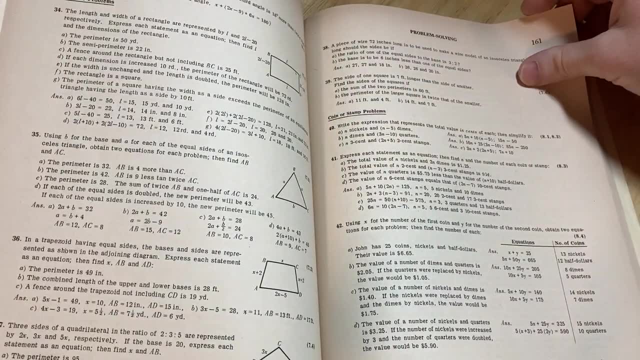 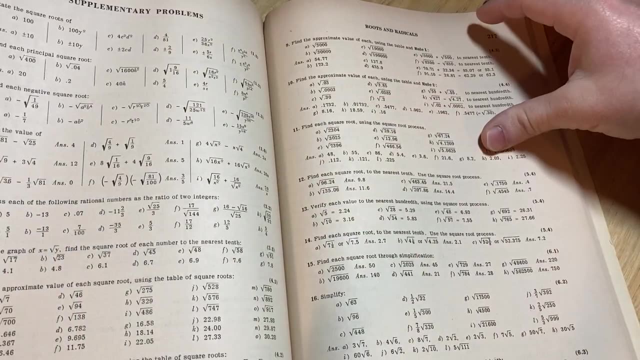 subsets, basically. so in a subset, you know, in sets, the order in which the elements are picked doesn't really matter. this is pretty cool, pretty cool book. here is wanted to show you one of my books. oh, here's the. you answers to supplementary problems. Oh, from, I guess we're. we're figuring out, like you know. 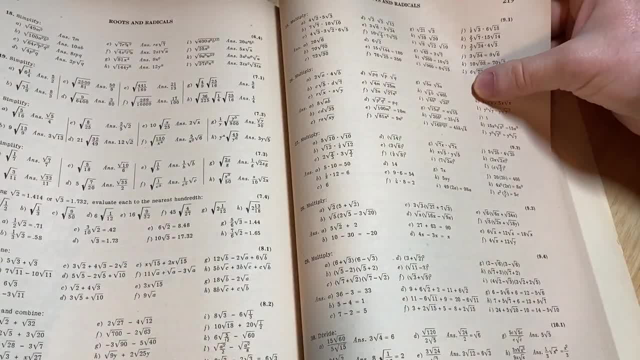 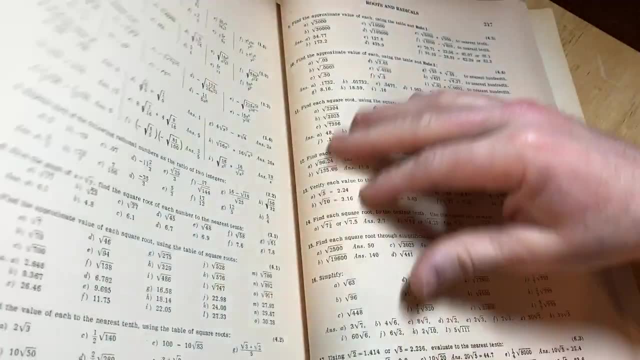 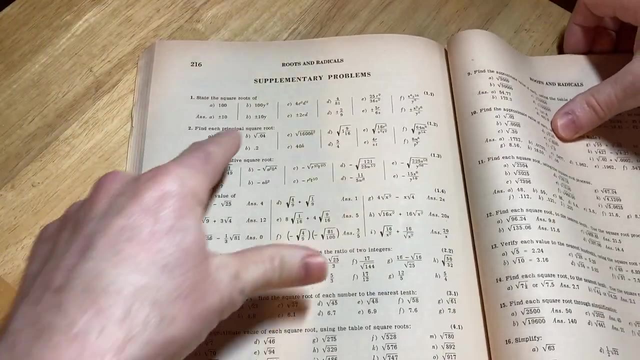 guess roots and radicals. Wow, Wow, Look at that Right, Tons, tons. So I guess, in that case, they. So here's the supplementary problems. Oh, here's the ones you actually have to do: State the square roots of 100.. Oh, there's the. 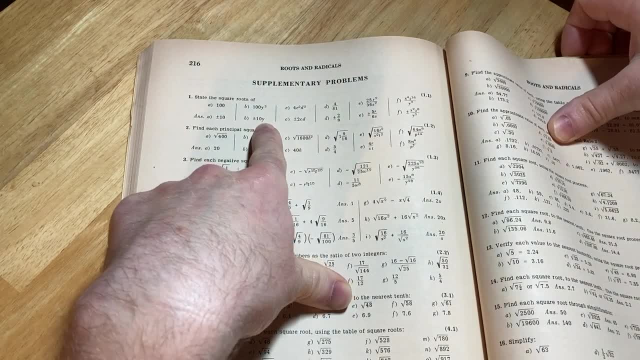 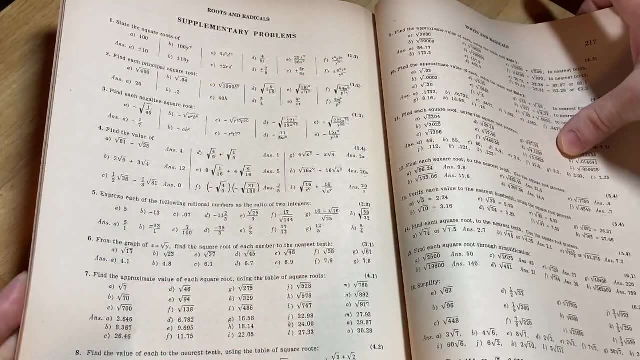 answer: right there, 100y squared, Boom. I like how they put the plus or minus there. on the y, It's important. the plus or minus, That's key. They're teaching good mathematics here, right? That's what this is. This is good. I gotta give it. 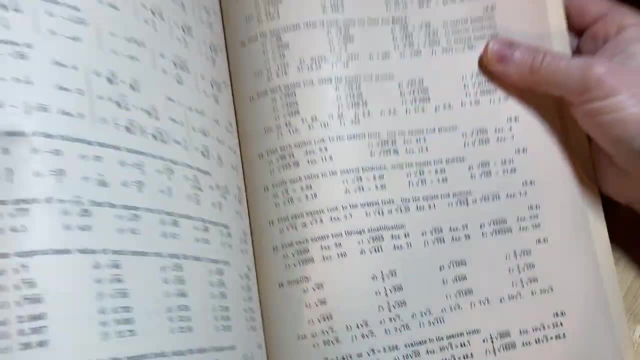 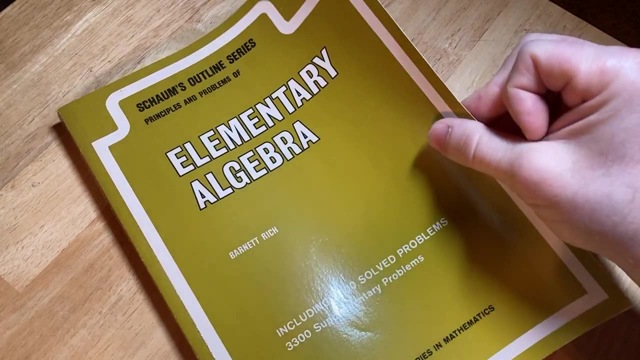 one more whiff, One more whiff. Yeah, really cool book here. Really like it. It's just a really fun color. Yeah, I like it. If you found any value in this content, feel free to hit subscribe if you want to. If not, that's cool too, I do have.